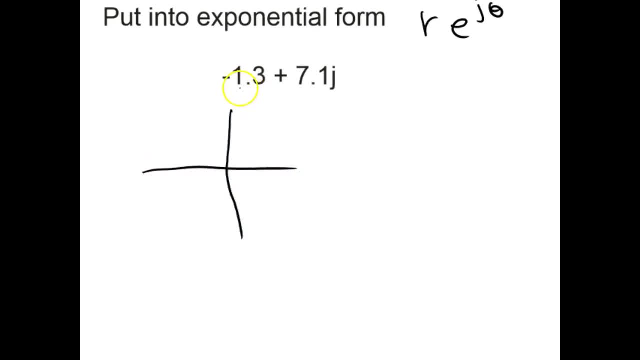 rectangular part. So negative 1.3. we would go this way: 7.1. we go up and this little line- here is my hypotenuse, is my r, and that's the theta we can find from our triangle To find r. it's the. 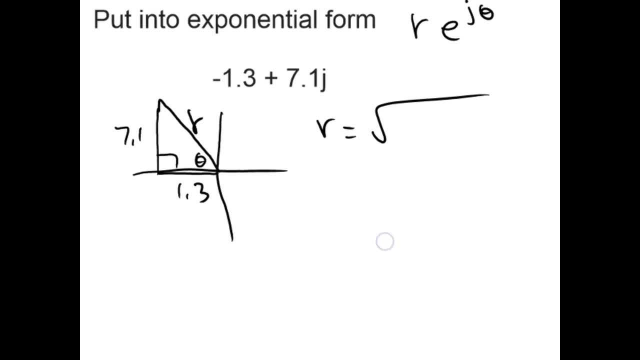 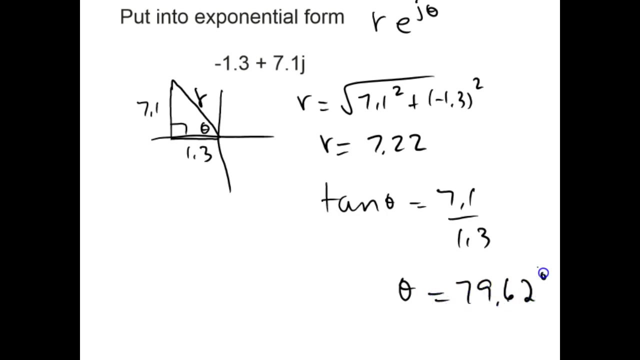 square root of- sorry, square root of 7.1, squared plus negative 1.3.. So r would give me 7.22.. My angle, my angle would be tan, theta opposite, over adjacent. So my angle would be 79.62 degrees. 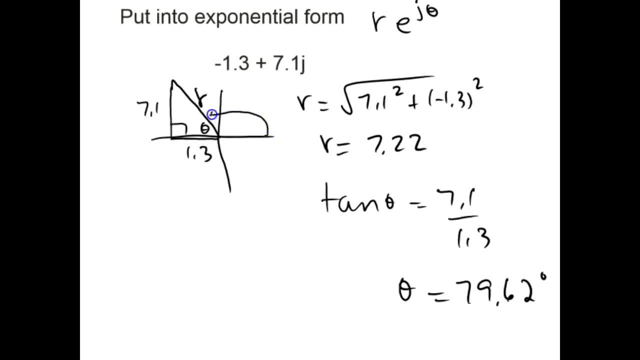 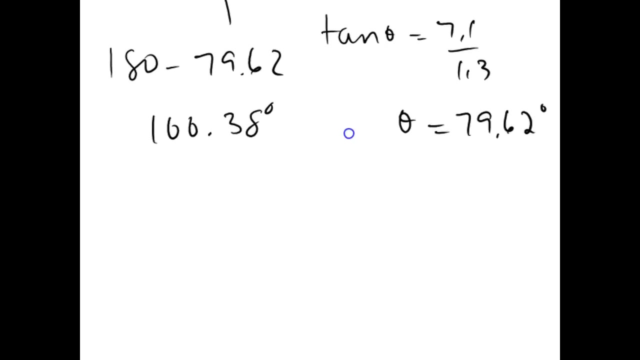 But that's not the angle I'm looking for. The angle I'm looking for is this one right here, We would get that by saying 180 minus 79.62, which equates to 100.38 degrees. So we can take our rectangular part and now change it into: 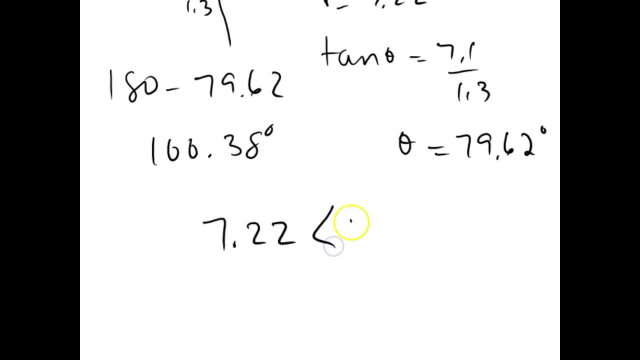 polar, which is 7.2, angle, 100.38 degrees. Now to change to that polar into rectangle- sorry, into exponential- we need to take our angle 7.2 and change into a radian measure. We do that by saying 100.38 times pi over 180. 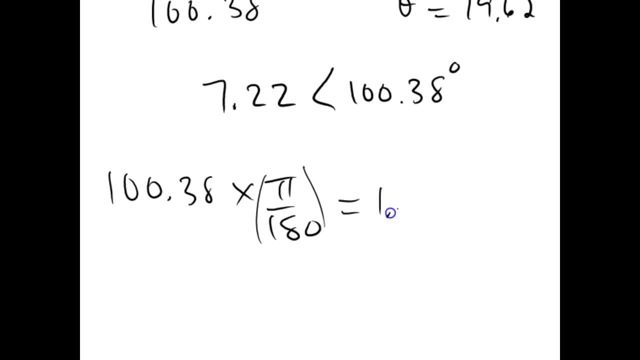 This gives us to four dozen points, 1.7520.. It's always important to have at least four dozen points. To put it into exponential form, we take our r value 7.22 e to 1.7520 j, and now that's in exponential form. So we're going to take our r value 7.22 e to 1.7520 j, and now we're going to take our r value 7.22 e to 1.7520 j. and now we're going to take our r value 7.22 e to 1.7520 j, and now that's in exponential form.